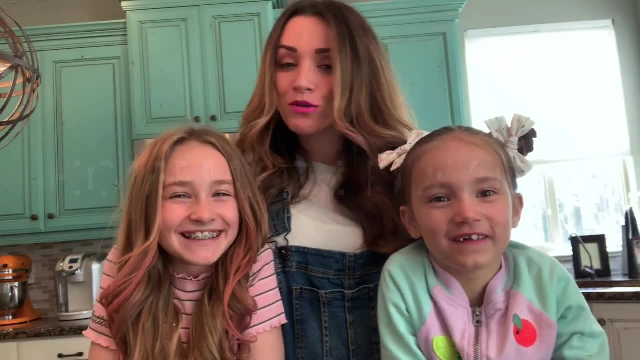 begging me to make what Play-Doh. So we're going to make Play-Doh, We're going to make it in three different colors and we're going to take you along with us, show you how easy it is to make Play-Doh. 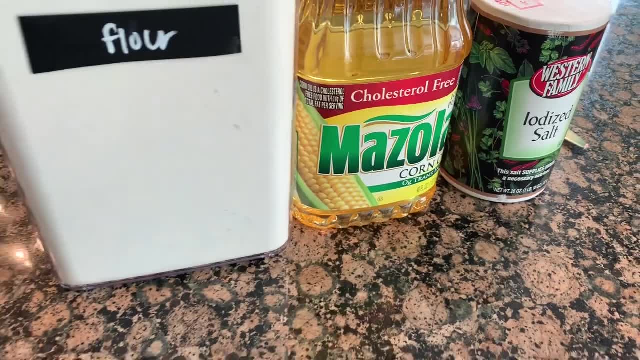 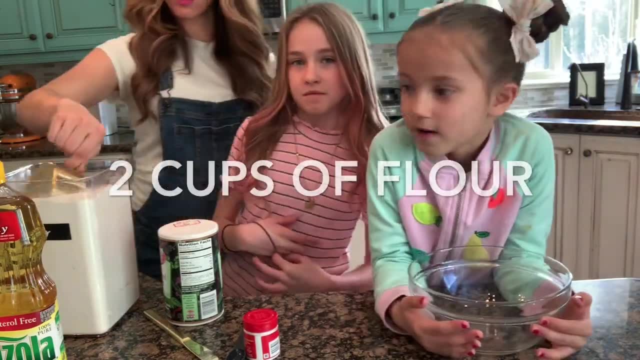 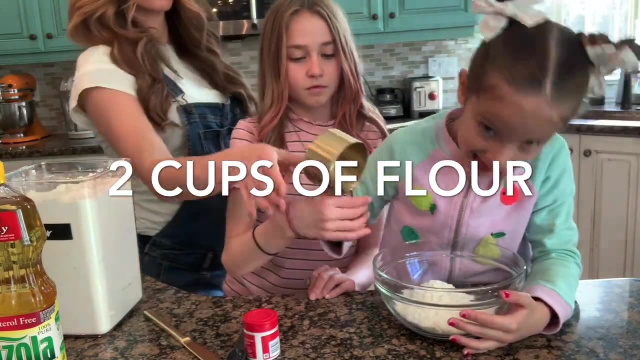 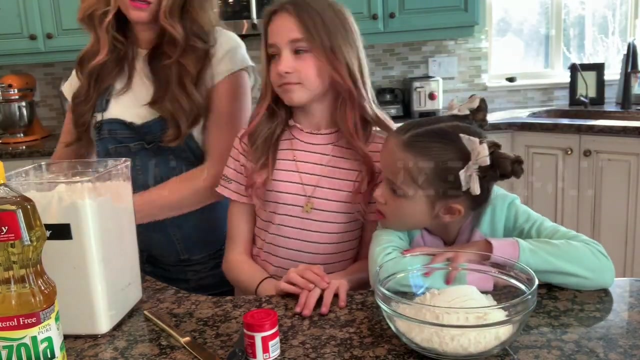 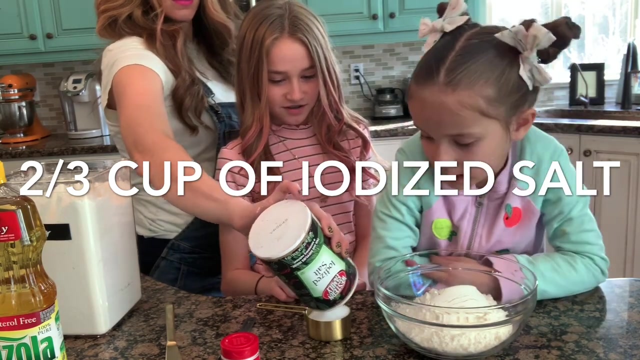 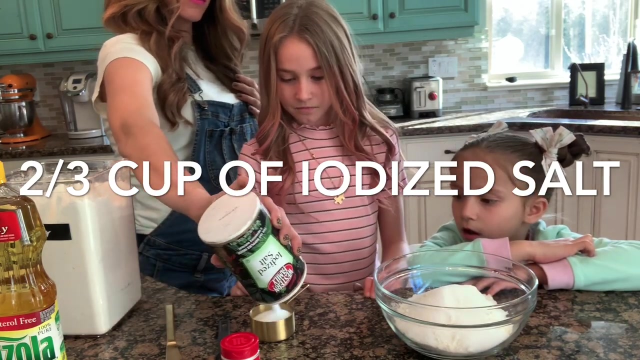 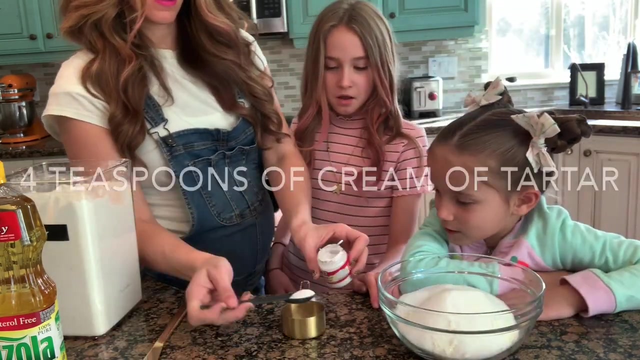 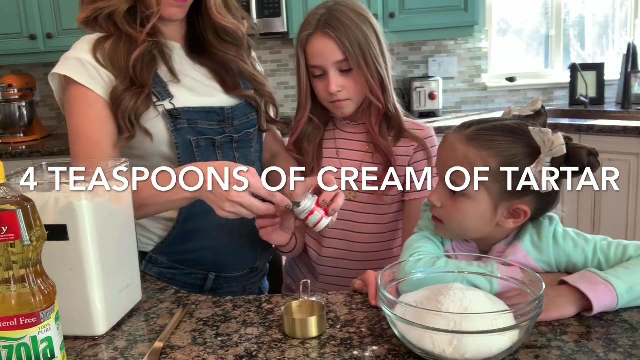 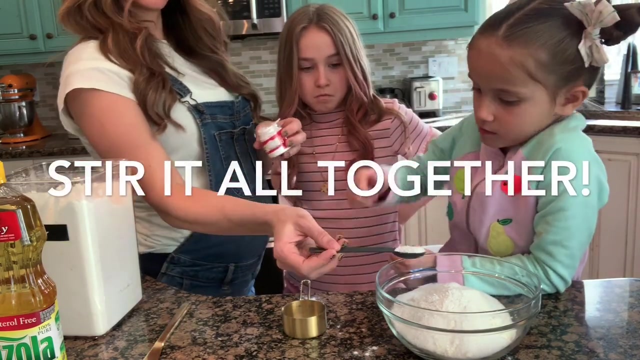 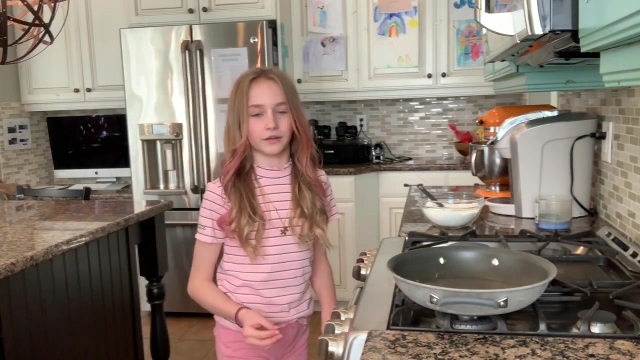 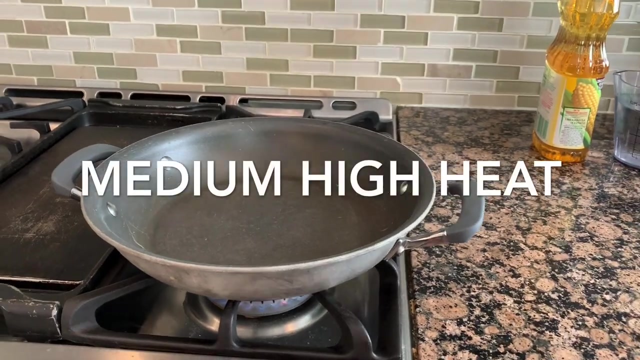 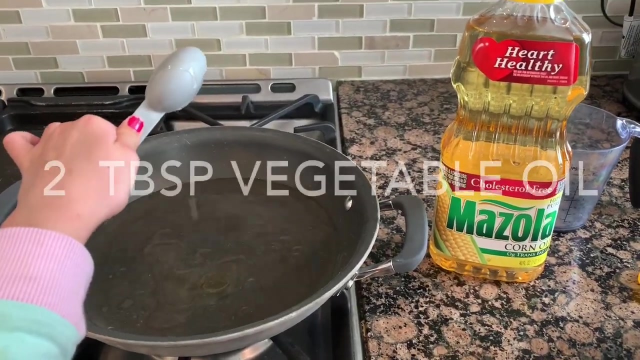 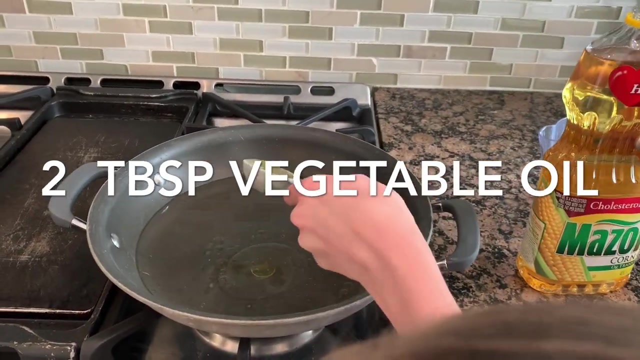 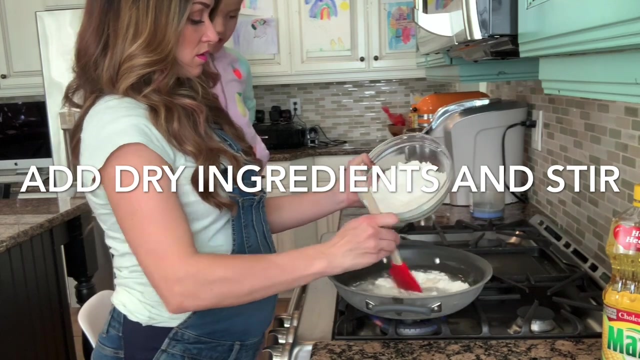 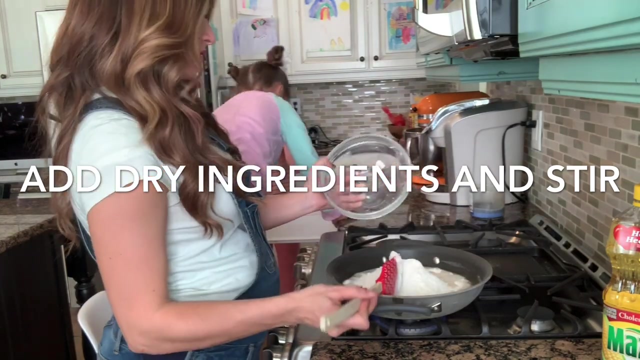 at home. Step one: put the dry ingredients into the bowl. So step two: now we're moving over to the stove and we're going to put our stove on to medium high heat. So now we're going to put the heat on and then we're going to turn up the heat. 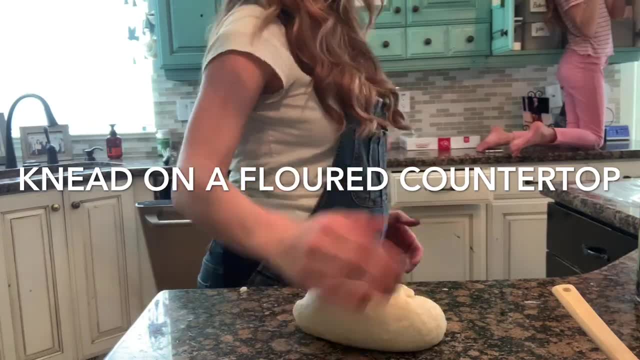 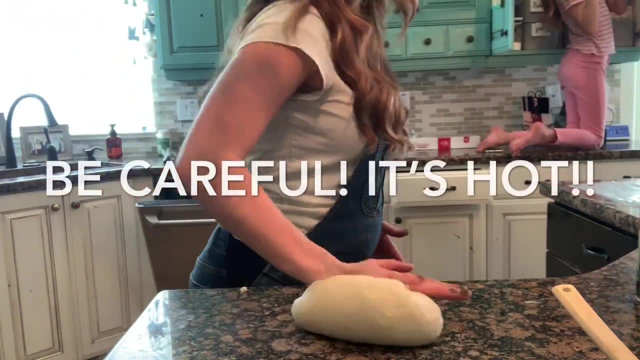 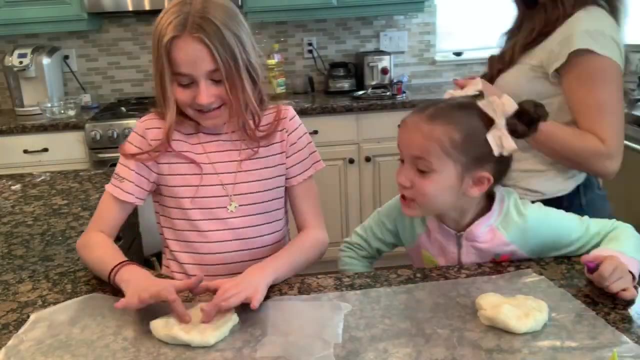 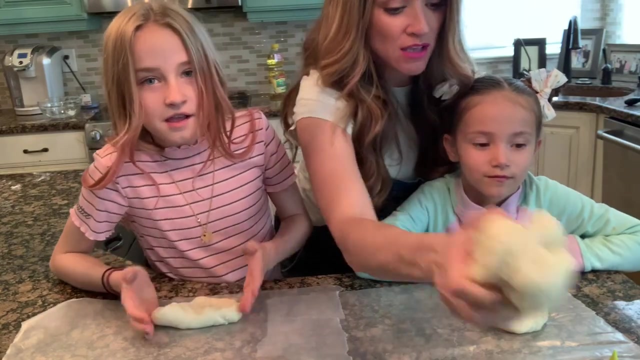 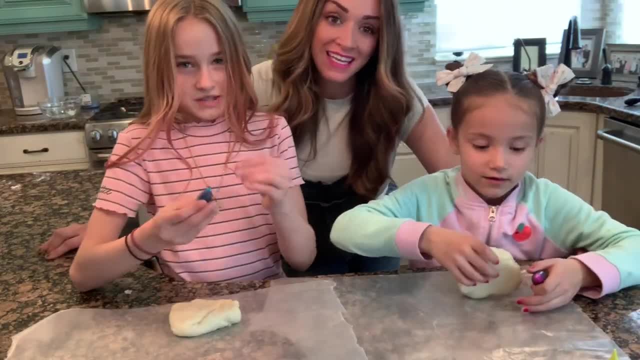 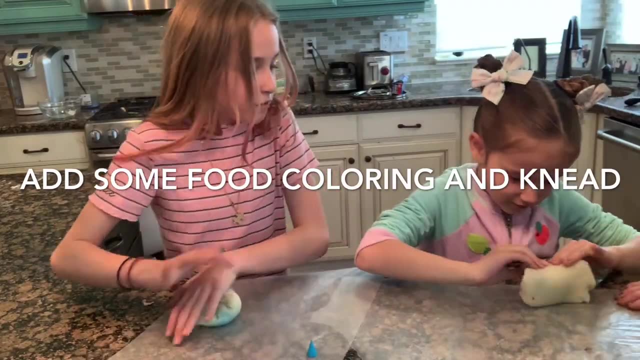 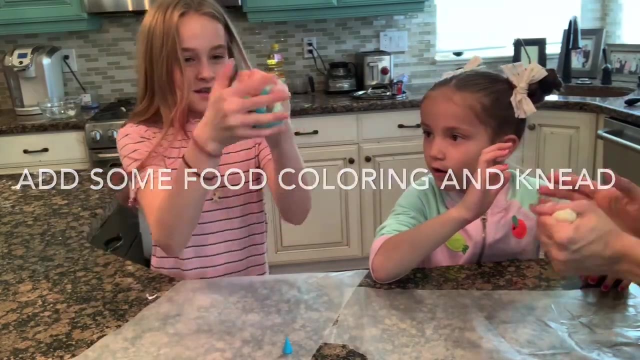 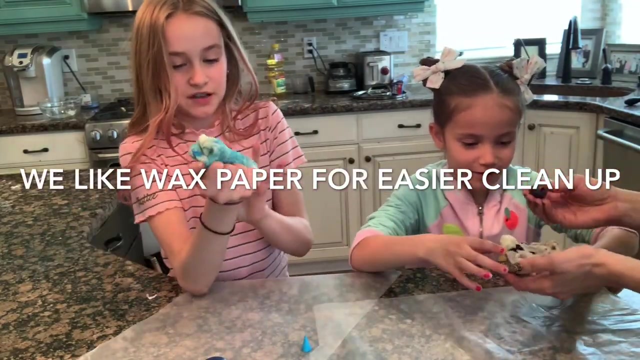 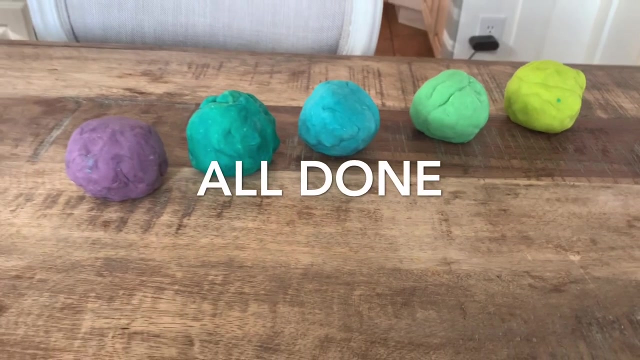 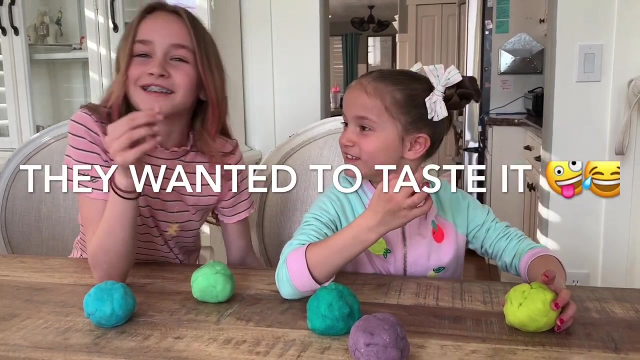 all you have to do is add a few drips of food coloring and then knead it in really, really well until the whole thing is colored. so so you ready, guys, Taste it Ready. I just licked it. Okay, ready, Yes, Go Go. Three, two, one Go. Let it sink in for a second.